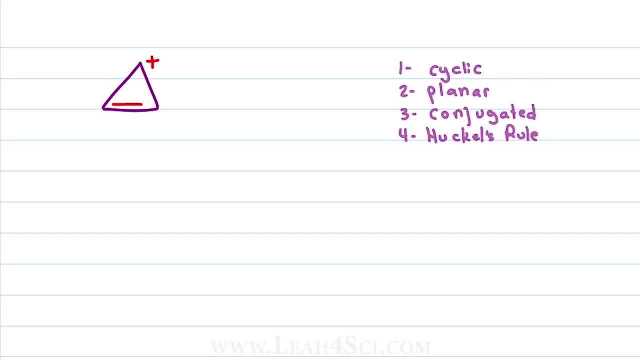 molecule with a pi bond and a carbocation. so let's break it down. How do we know if it's aromatic? The molecule is cyclic. I can trace a circle around the entire compound. It's planar because every carbon is sp2 hybridized. The carbon is holding the pi bond as well. 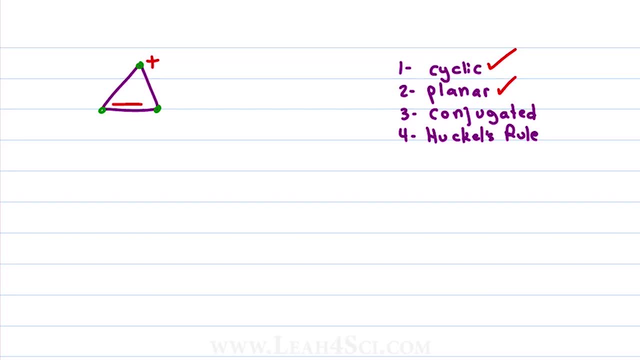 as the carbocation. We know that the pi bond can resonate into that MTP orbital either towards the left or towards the right. Let's call this a fully conjugated system, and then we'll use the shortcut for Huckel's rule. We have a total of one pi bond, which is odd, and odd number of pi bonds follows. 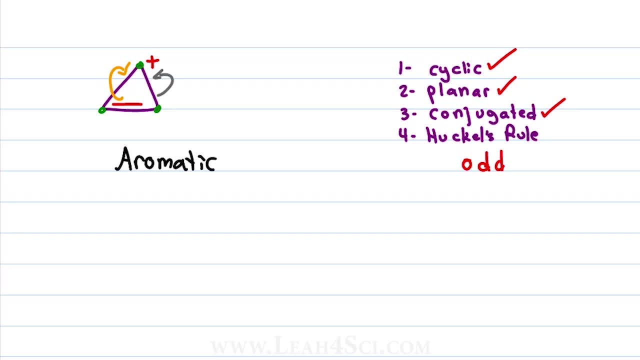 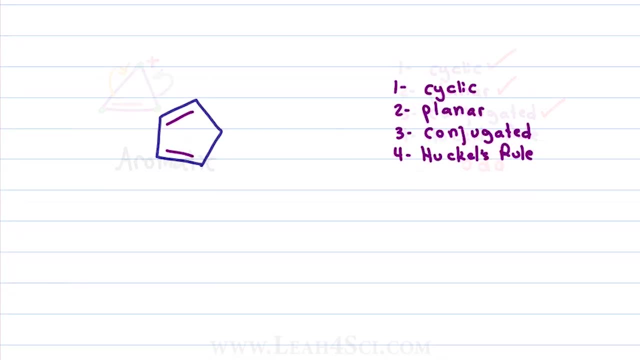 Huckel's rule making this molecule aromatic. Yes, it's tiny, yes, it's under a lot of strain, but it's still aromatic. We've seen that cyclopentadiene is non-aromatic because of an sp3 carbon atom. but what if? 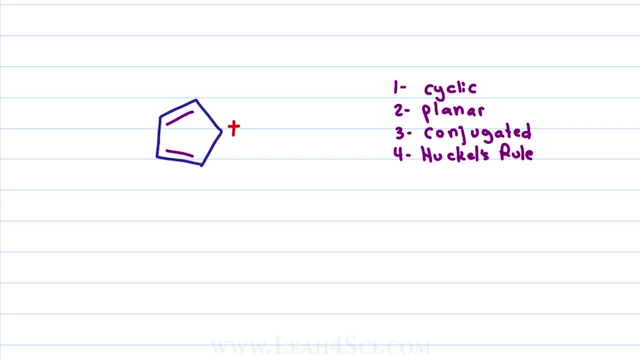 we change it To the cyclopentadienyl cation, meaning a positive charge on the carbon that doesn't have a pi bond. The molecule is cyclic. I can trace a circle from start to finish. The molecule is planar because every carbon atom in this ring is sp2 hybridized. The carbon is holding. 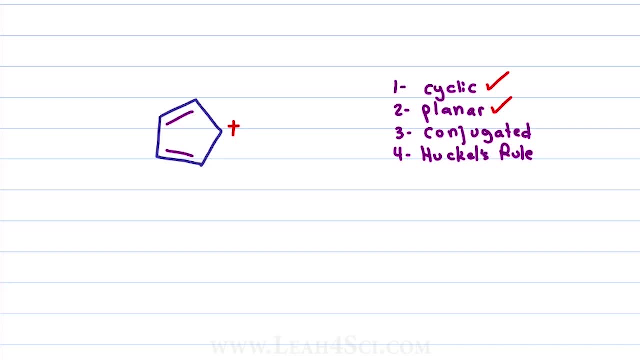 a pi bond and the carbon holding the carbocation. The molecule is conjugated because the pi bonds can resonate in the direction of the carbocation clockwise, But does it follow Huckel's rule? Let's see: We have a total of 4 pi electrons or 2 pi. 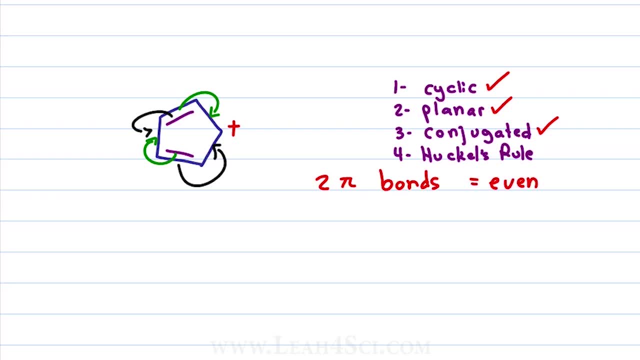 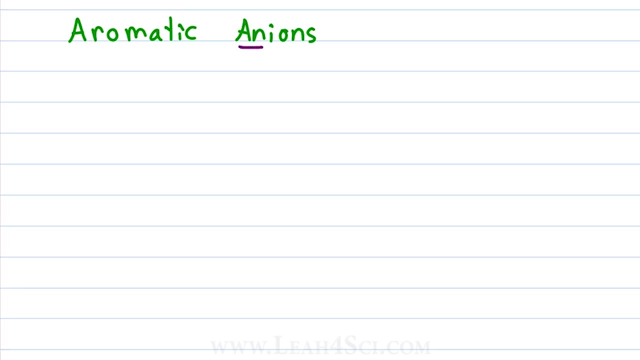 bonds. That means we have an even number of pi bonds and even does not follow Huckel's rule. It's anti-team. Huckel making it anti-aromatic. Aromatic anions are evaluated the same way, with one difference: An means without. but 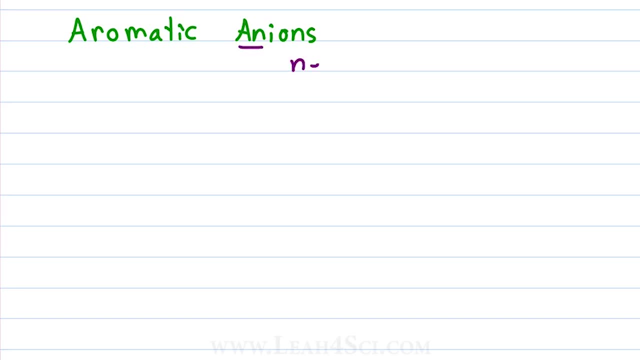 in this case, it means without an ion. It means that an ion is not an ion. It means that an ion is not an ion. It means that an ion is not an ion. It means that an ion is without or negative, because we're dealing with a negative charge. 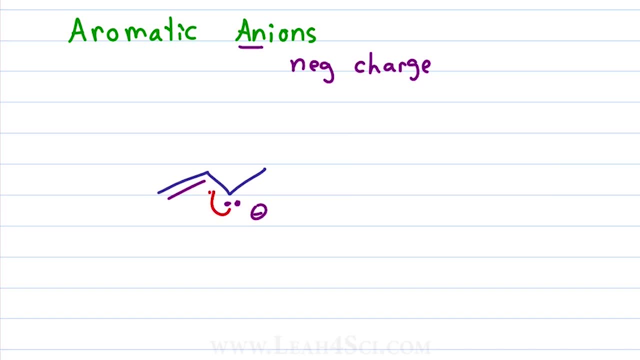 If we have a system with a pi bond next to a carbon ion, the negative electrons can resonate towards the pi bond, kicking those electrons, which gives me a resonance structure that now has a pi bond in the middle and a lone electron pair on the left, definitely capable. 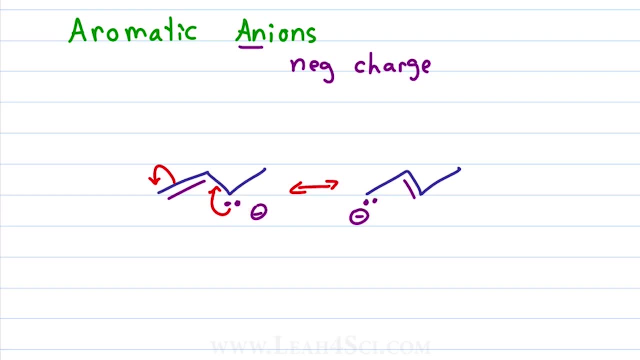 of resonance. In order for these electrons to resonate, the carbon has to hybridize to sp2.. We're going to take the lone electrons into a p orbital so that it can participate in the resonance, and this is something to keep in mind when evaluating the aromatic anions. 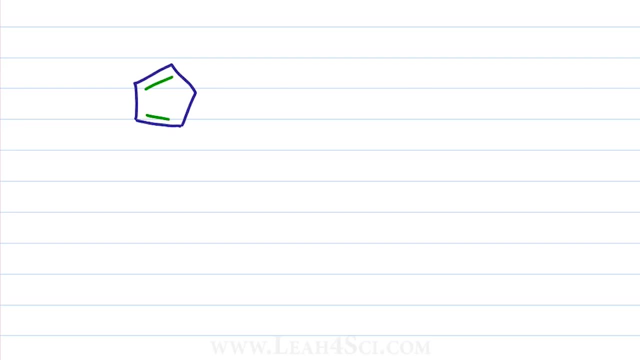 We'll take our same cyclopentadiene, but this time we'll give it a lone pair rather than a carbocation on this carbon atom, which means it also has a negative charge. Let's evaluate. We already know that it's cyclic, because these electrons can resonate. 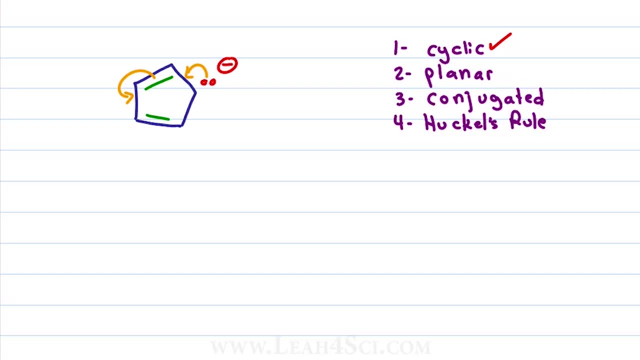 towards the pi system. They have to sit on an sp2 hybridized carbon atom, which means all of the carbons are sp2 and the molecule is planar Because the anion can resonate into the ring. that makes it a conjugated system, but does it follow Huckel's rule? We? 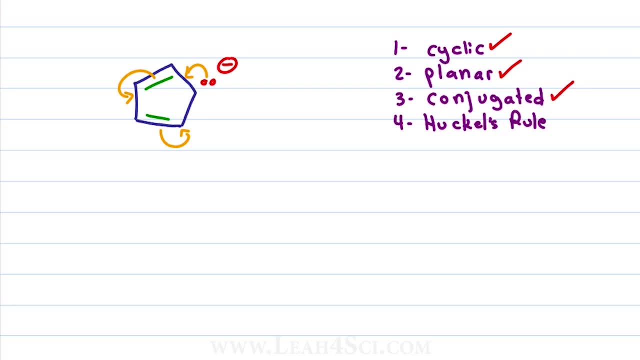 have two pi bonds, which means an even number. but remember that for Huckel's rule we're not looking at the number of pi bonds as much as the electrons that are resonating or, the short cut, the electron pairs that are capable of resonance. We have a total of 6 electrons. 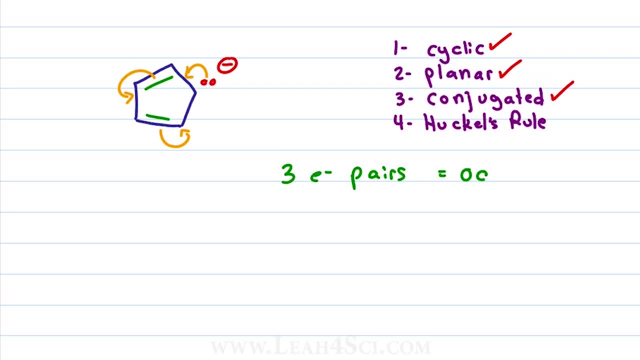 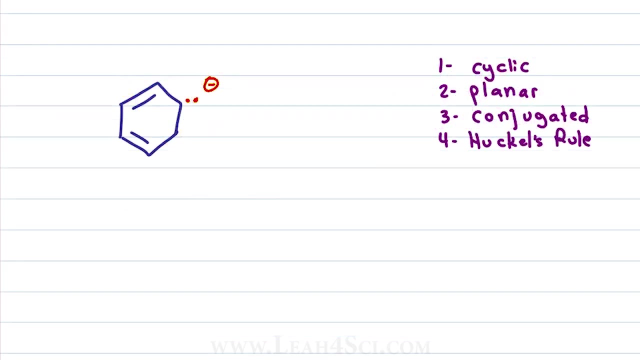 or 3 electron pairs, which means we have an odd number. and an odd number means it follows Huckel's rule. That makes the cyclopentadieno anion an aromatic anion. Let's compare to this 6 carbon anion. The molecule is cyclic, because I can trace a path. 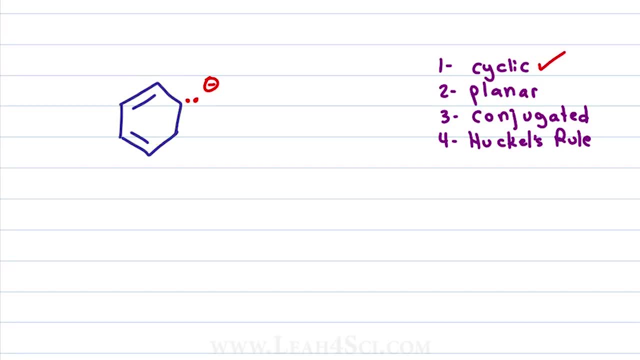 around the ring, If you notice the anion, which means, if my mind jumps to Huckel's rule, I'm thinking: 6 electrons, 3 electron pairs, odd number should be aromatic. but what else do we have going on? Yes, the negative electrons can resonate into the ring, making part of the 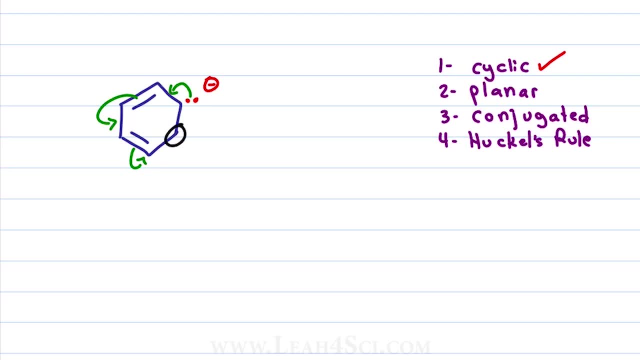 system conjugated, but don't forget, we also have this carbon over here. This carbon is not able to participate in resonance because it doesn't have a charge and it doesn't have a pi bond. It's an sp3 hybridized carbon, meaning it's tetrahedral or 3-dimensional. That means the 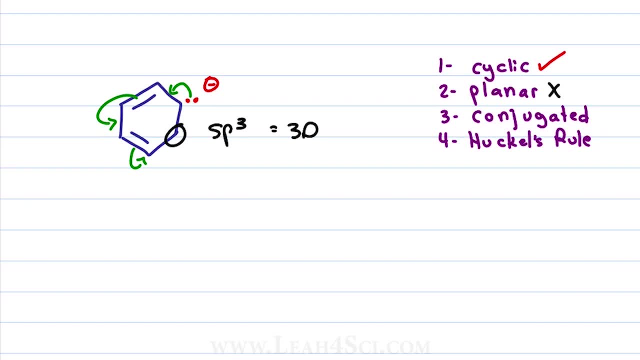 molecule is not going to be planar and the entire ring is not conjugated because we can't resonate onto sp3. This sp3 carbon is uninterested in aromaticity, is a non-baseball fan, making this a non-aromatic compound. Let's move on to heterocyclic aromatic compounds, Remembering 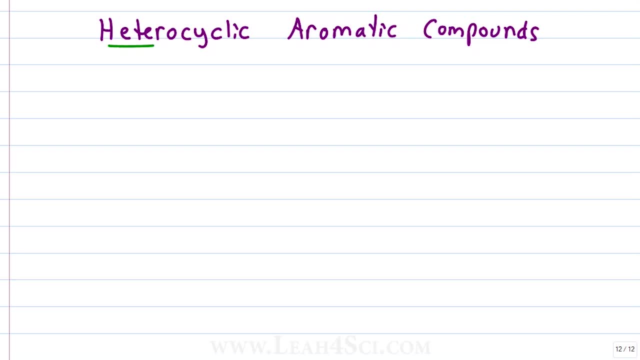 that hetero means non-aromatic compound and heterocyclic means non-aromatic compound. Heterocyclic means different, and a heterocyclic compound is a molecule that has something different in the ring, meaning other than carbon atoms, For example, this molecule right here: 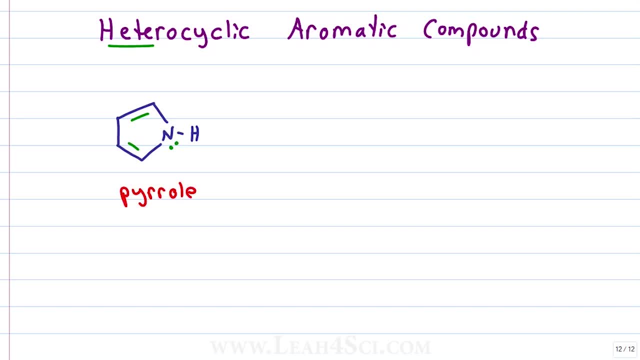 often comes up on exams: Is pyrrole an aromatic compound or not? More importantly, how do we evaluate when we have something like a nitrogen atom in the ring? Here's the trick to remember with heterocyclic compounds. Heterocyclic compounds are very stable, so when possible, everything wants to be stable. 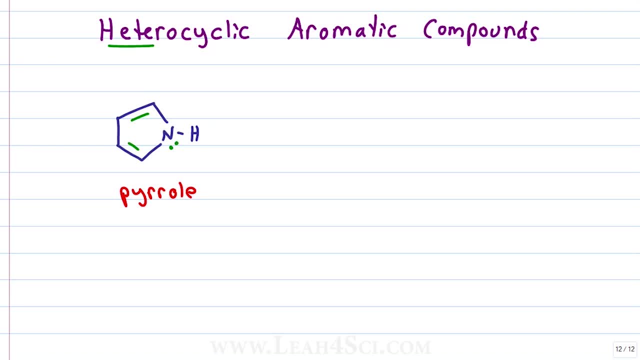 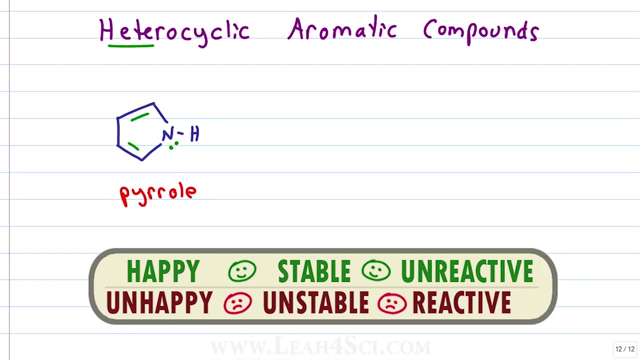 This is something that you'll hear me say over and over and over. It applies to organic chemistry just like it applies to your entire life. Happy is going to give you. something that is stable is going to be unreactive. If something is unhappy, it is unstable, and 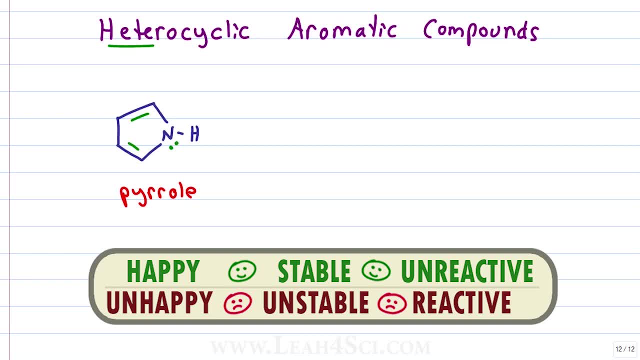 that makes it reactive. We said that aromatic compounds are very stable, so, when possible, everything wants to be aromatic. if it can, A heterocyclic atom, if it has the ability, will try to contribute to aromaticity. But in order to be aromatic it has to resonate. so here's the question to ask. 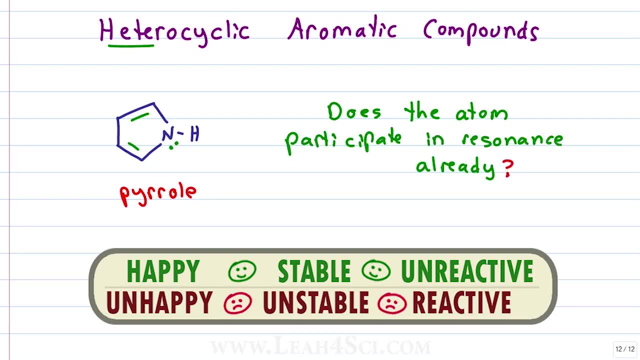 Does the atom participate in resonance already? All you need is one participation. An atom can't join resonance with two separate electron pairs at the same time. It's one pie bond, one lone pair. that's it. If the atom is already participating with a pi bond, you don't add the electrons in. 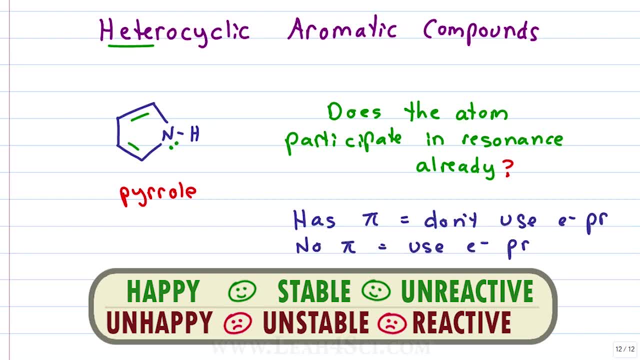 If the atom is not participating, you use the lone pair. Again, if the atom has a pi bond, you don't use its electron pair. If it has no pi bond, you use its electron pair. If it has two electron pairs, you only need one, because one is enough to participate. 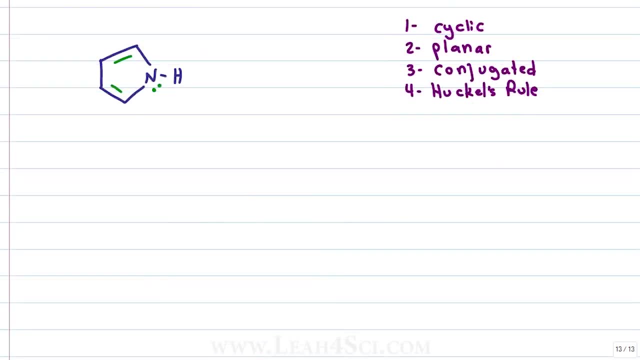 Let's see how this applies to pyrrole. Is the molecule cyclic? Why, yes, it is. I can draw a circle around the ring, including the nitrogen atom. Is the molecule planar? Let's see The carbons have pi bonds. they look sp2 hybridized. 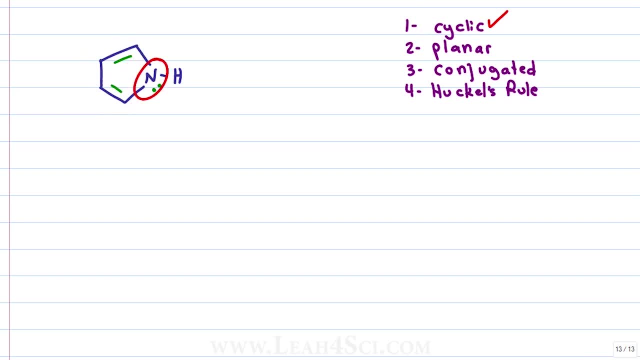 The nitrogen atom appears to be sp3 hybridized. It's got three bonds, one lone pair which would sit in a hybridized orbital. except for the rule you should remember from resonance- and I cover this in the series Link below- If the atom has the ability to resonate, then it will hybridize so that it can resonate. 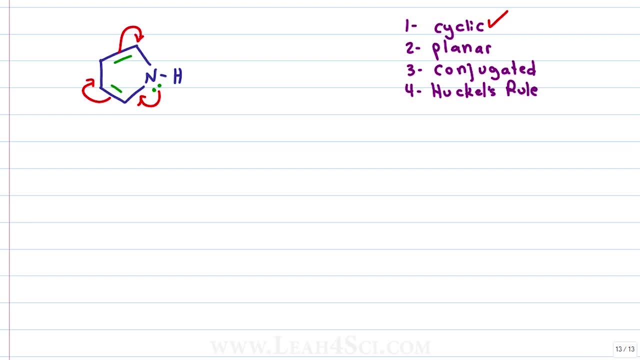 That means, even though nitrogen appears to be sp3, the nitrogen is sp2, hybridized so that it can participate in resonance, which means the molecule is planar, everything's resonating, and it means the molecule is conjugated. But do you notice how we had to ask the question? 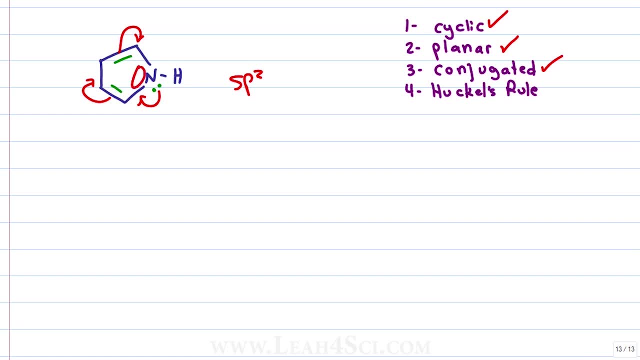 Nitrogen. Yes, it's not a ana And Helen's No sitting above and below, so we'll draw above and below in two different colors and then we have a nitrogen atom right over here. If nitrogen is sp2 hybridized, that means it's going to have 120 degree bond angles between. 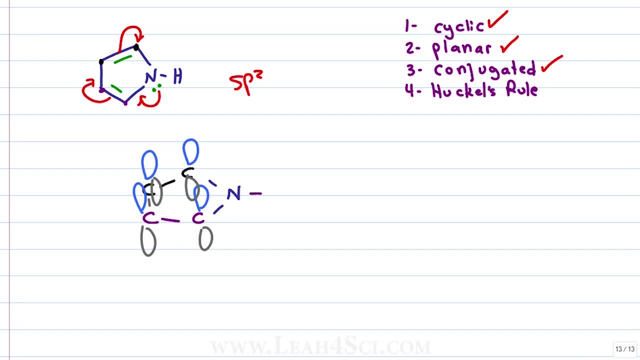 nitrogen and the things it's bound to. that puts hydrogen perpendicular to this system facing completely out of the way. But then we have that p orbital where the electrons would sit. we've seen that we have a pi bond here and here like this, but now nitrogen can take those electrons resonate. 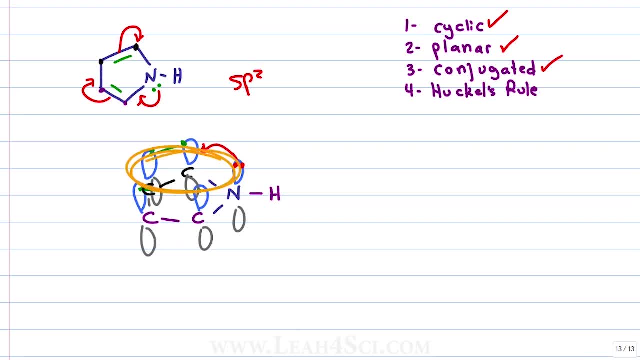 towards the pi bond. giving me that conjugated system, Let's verify with Huckel's rule: how many electron pairs do we have? Two pi bonds and one lone pair gives me a total of three electron pairs, an odd number of electron pairs, which means it supports team Huckel and it's aromatic. 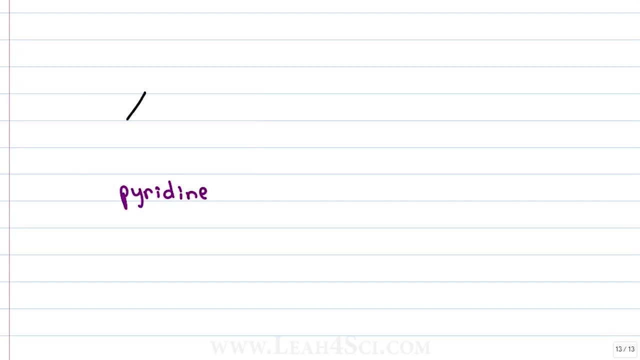 Another common molecule you'll see Is pyridine. pyridine, like pyrrole, is a heterocyclic compound that appears to be aromatic. Let's take a look. Is it cyclic? Yes, it is. Is it planar? I see pi bonds everywhere. all sp2 hybridized? yes, it is. 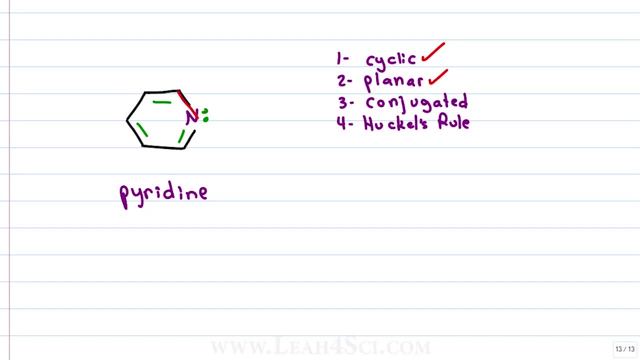 Is it conjugated? It looks very much like benzene. in fact, if I pretend the nitrogen isn't there, it's exactly benzene, which means it is conjugated. But what about Huckel's rule? I have three pi bonds and one lone pair, giving me a total of four electron pairs, or an even. 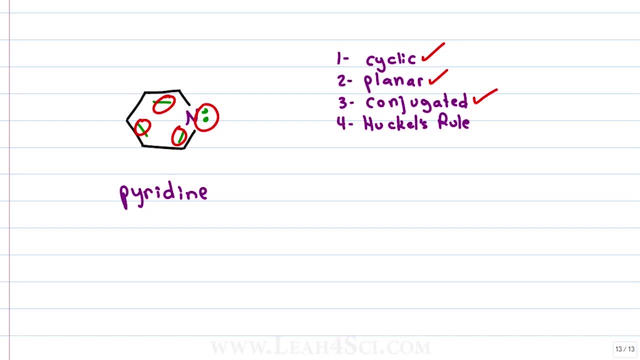 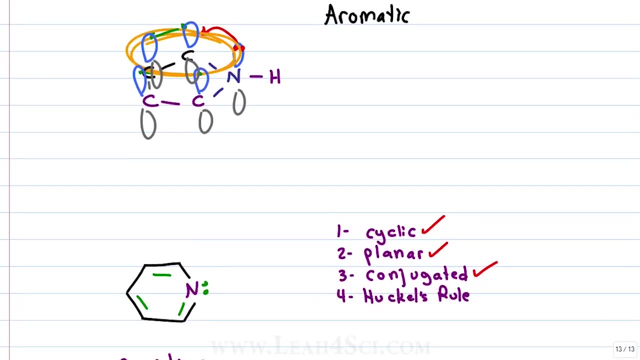 number which wants to tell me that the molecule is anti-aromatic. We have to go back to the rule: Nitrogen wants to participate in aromaticity. in pyrrole, the only way to play was to bring its own electrons. BYOE, bring your own electrons, but in pyridine we don't need that because 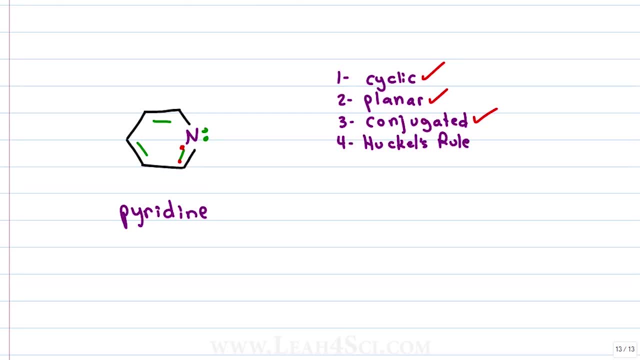 nitrogen already has a pi bond. it's already part of the resonating system. That means these electrons don't get to play along. therefore they're not counted, and so we have one, two, three. an odd number of electron pairs. supports team Huckel making. 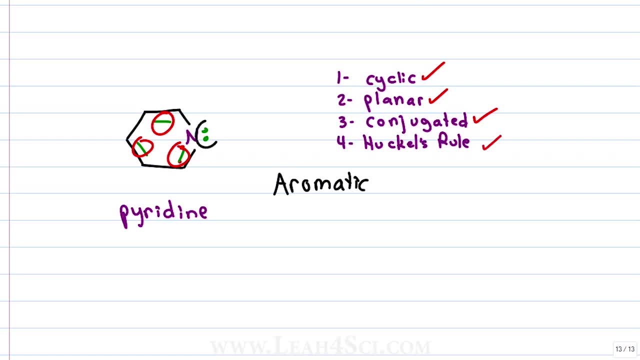 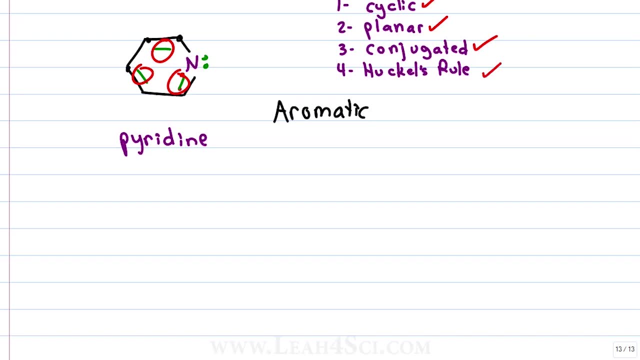 pyridine aromatic. Let's take a look at a side view so you understand why these electrons can't even try to participate. We'll show these three carbons in black And the forward carbons in purple and nitrogen. on the side, We'll show the upper part of the p orbital in light blue, including on nitrogen and the. 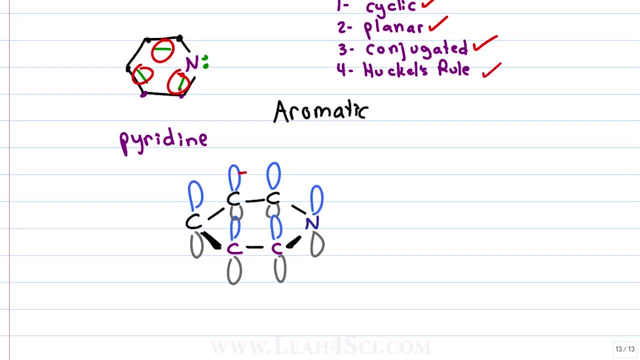 lower part in gray and look what happens. We have a pi bond here, we have a pi bond here and we have a pi bond here. That is a clearly resonating system. but what about the lone pair If nitrogen is sp2 hybridized? 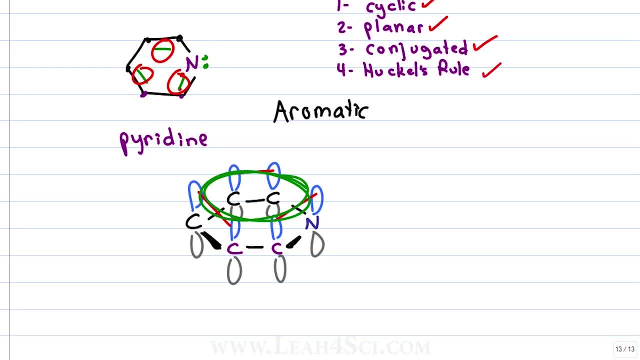 Then imagine that this lone pair is sp2 hybridized. This lone pair is really a bond to itself in an orbital that sits at 120 degrees perpendicular to the molecule. Even if these electrons wanted to participate, they're sitting at 90 degrees.